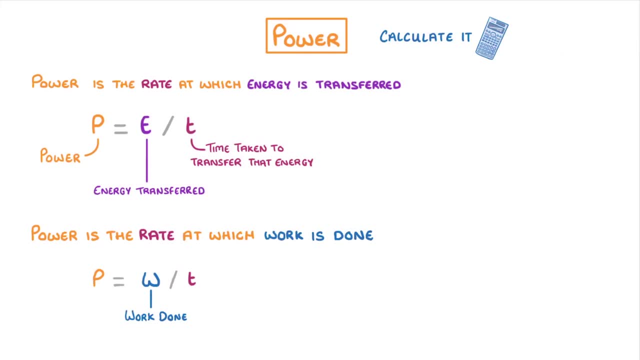 can be a bit confusing, but basically it's just a special measure of the energy transferred and is used when a force is used to move an object by a certain distance. For example, if you pushed a car down the road, then the energy that was required would. 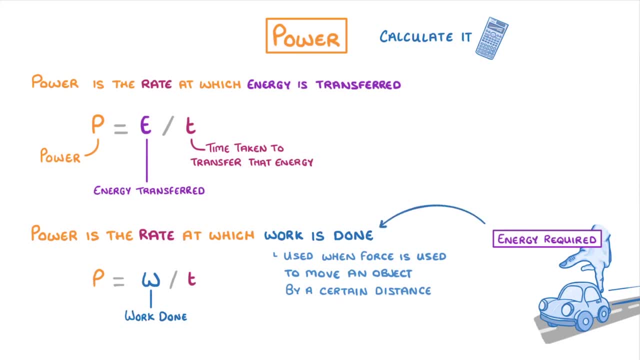 be referred to as the work done, as you moved it a certain distance, Whereas if electrical energy was transferred from a plug socket to your phone, we'd refer to that as just energy transferred, as there's no force or movement involved. In both cases, though, power is measured in watts. energy transferred and work done are. 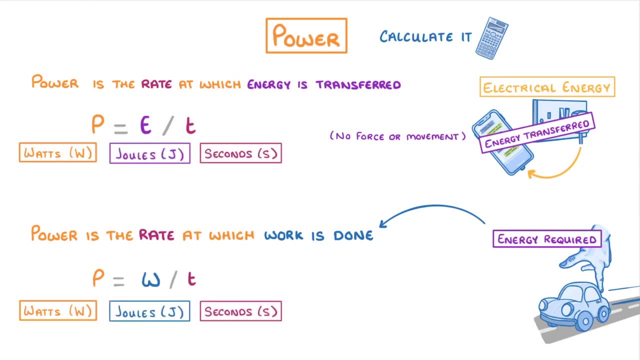 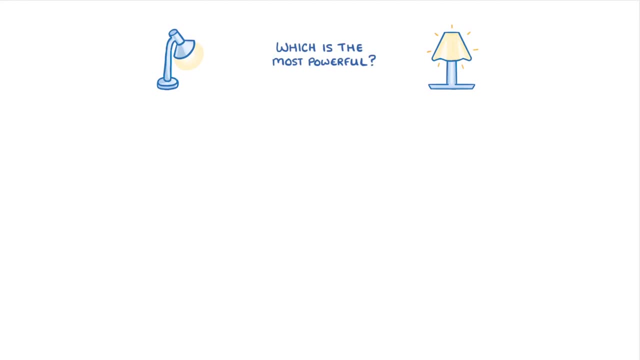 measured in joules and time is measured in watts. To see how the equations work, let's compare two lamps to see which of the two is most powerful. The lamp on the left transfers 1200 joules over 20 seconds, while the other one 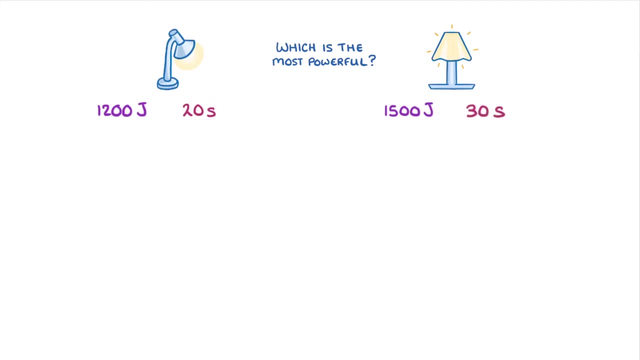 uses 1500 joules over 30 seconds. In this case, we'd be using the energy transferred version of the power equation. as there's no work being done For the left lamp, we'd do 1200 joules and then we'd use the second lamp to see which of the two is the most. 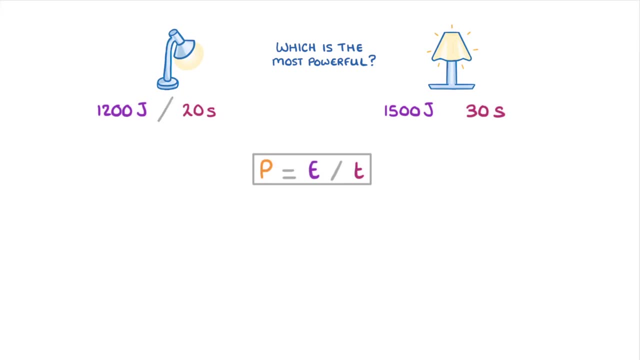 powerful, divided by 20 seconds to give us 60 watts as the power. And for the right lamp we'd divide 1500 joules by 30 seconds to give 50 watts, So we can tell that the left lamp is more powerful. 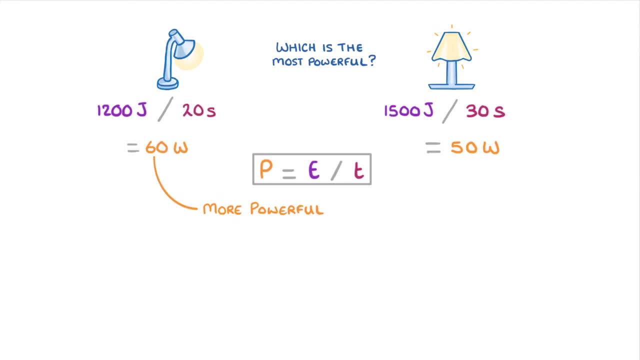 If you look on your lamp at home, there may well be a label telling you its power. Let's now try a slightly harder example. If an 1100 watt microwave is on for 3 minutes, how much energy is transferred? First, we need to take our energy transferred equation and rearrange it to get energy transferred by itself. 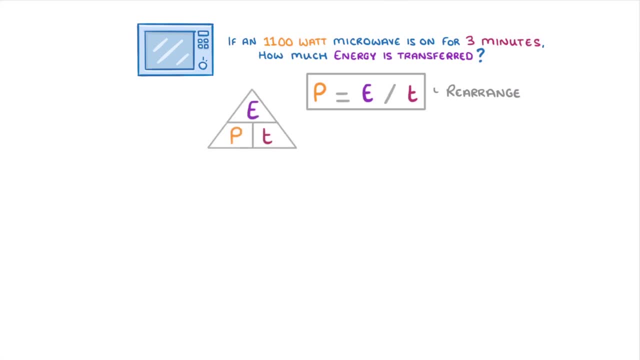 If we put the equation into a formula triangle like this, we can see that energy transferred would be equal to power times time. We also need to change our 3 minutes to 180 seconds by multiplying it by 60. And finally, we can substitute our values into the equation and do 1100 times 180, to give us 198,000 joules.